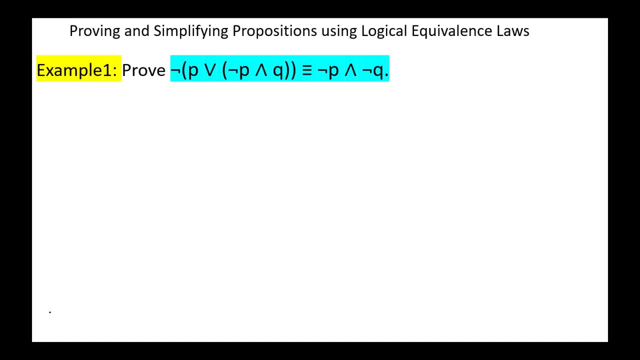 Example 1. We obtain not P disjunction, not Q, which is equivalent to not P conjunction P, by using double negation law- disjunction, not Q- And by using distributive law. this is equivalent to not P conjunction. 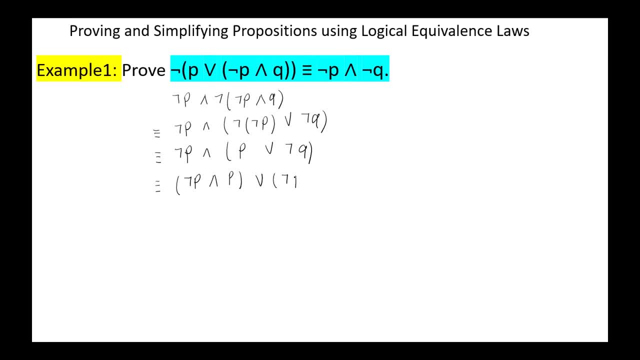 Conjunction P disjunction, not P conjunction, not Q. Using negation law, not P conjunction. P is always false Disjunction, not P conjunction, not Q False disjunction. R is equivalent to R, So this is equivalent to, not P. 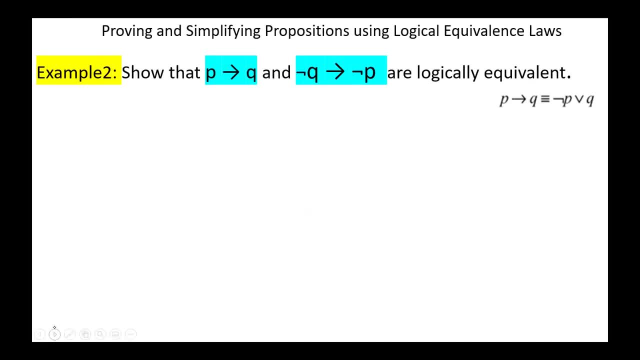 Not Q. Hence approved Example 2.. Show that P implies Q and not Q implies not P are logically equivalent By definition. P implies Q is equivalent to not P. disjunction Q: The right side: not Q implies not P is equivalent to not not Q. 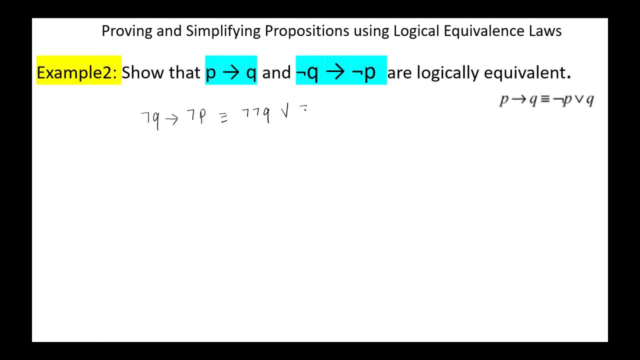 False disjunction, Not P. By using double negation law, this is equivalent to Q disjunction, not P. And by using commutative law, this is equivalent to not P disjunction Q. The same as P implies Q. 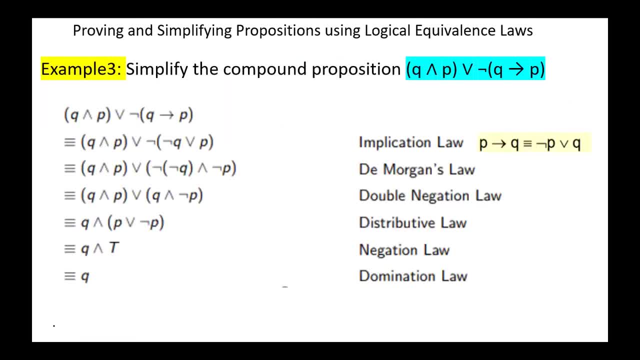 Hence approved Example 3.. Simplify the compound proposition: Q conjunction P, All disjunction, not in parenthesis. Q implies P. Here we have the original expression. This is equivalent to Q conjunction B, disjunction not, not Q disjunction B. 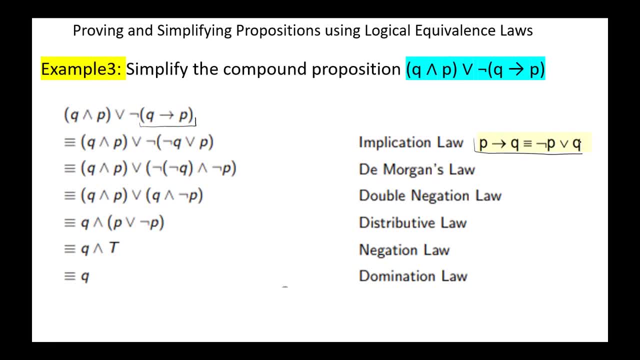 This part is obtained from the implication law And this is equivalent to Q conjunction, P disjunction. By applying demoralization We obtain not, not Q conjunction, not P. Q negated twice is Q. So this is equivalent to Q conjunction, P disjunction. Q conjunction, not P. 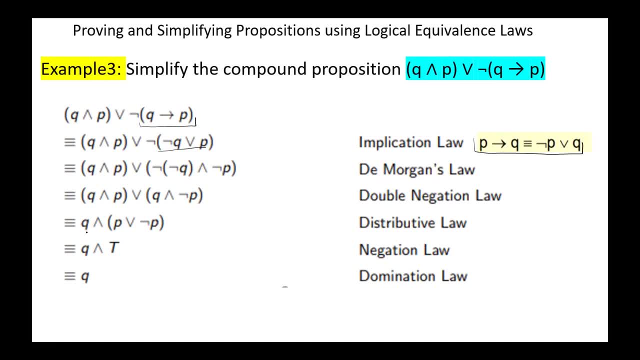 By applying distributive law we obtain Q conjunction, P disjunction not P, B disjunction not P is always true. And the last simplification, Q conjunction is true, equals to Q. So this compound proposition is simplified to Q. 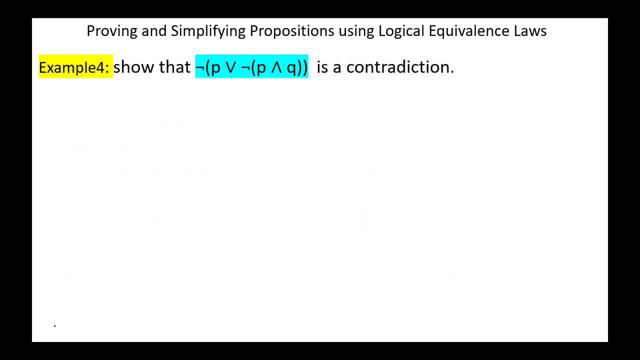 Example 4. Show that negation of P disjunction, negation of P conjunction Q, is a contradiction By applying De Morgan's law, this is equivalent to not P conjunction Q, Not not P conjunction Q, which is equivalent to not P conjunction by using double negation. 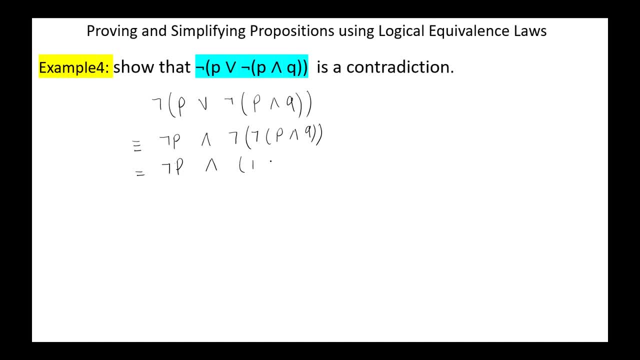 we obtain here P conjunction Q, And this is equivalent to by applying distributive law. not P conjunction Q, Not P conjunction P is always false, So this is equivalent to false conjunction Q. 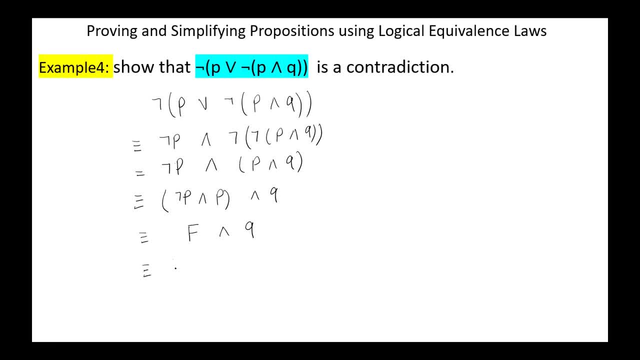 False conjunction Q is always false, Which means that the compound proposition is a contradiction. Hence proved, And the last example for today Show that the following implication is a tautology, not our conjunction: are the junction s implies s. first, we use the implication.